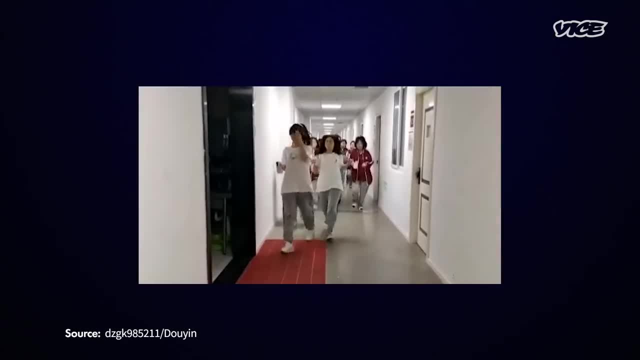 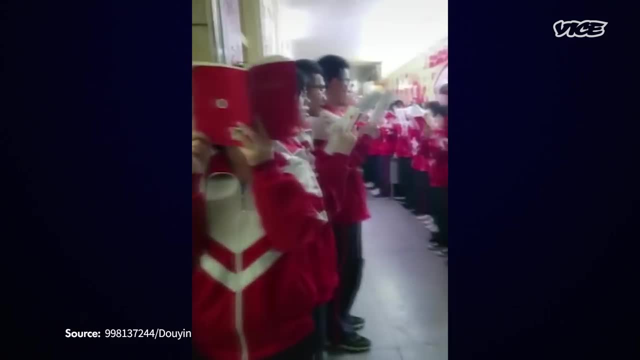 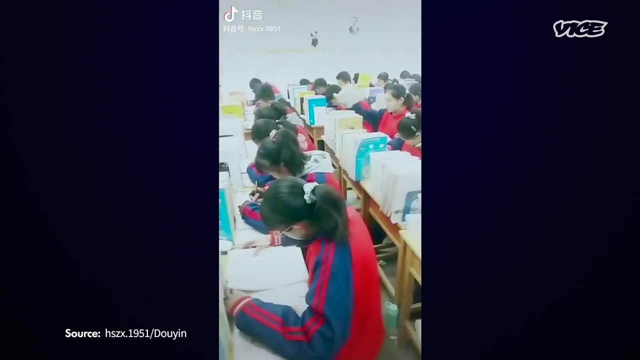 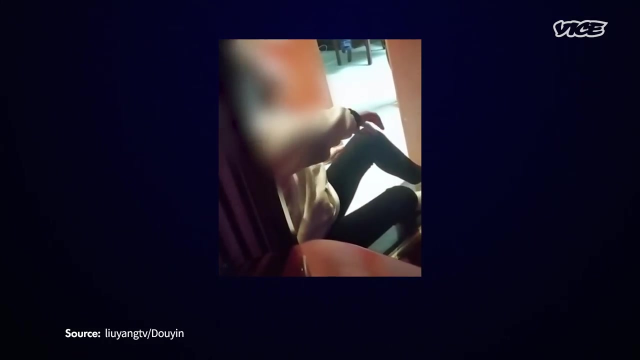 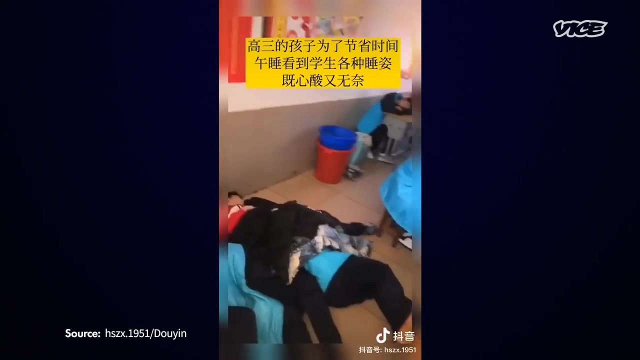 Wake up before sunrise, sleep after midnight. It's a typical day for students who are prepping for China's most competitive exam, the National College Entrance Examination. This obsession with good academic performance is ingrained in parents and students of all ages, but it's taking its toll on many students' mental health. 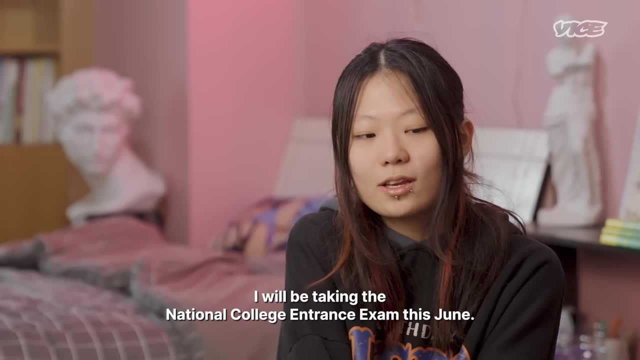 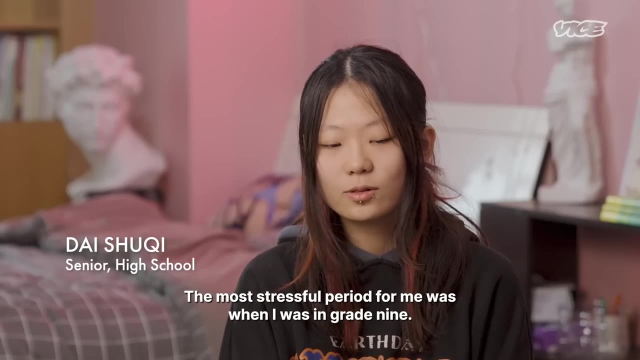 I was 18 years old this year and I took the college entrance exam in June this year. I think I was the most stressed out when I was in the third year of junior high school. That year I was sent to a tutoring school. 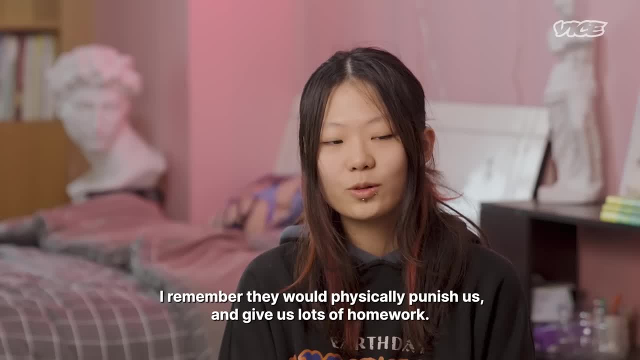 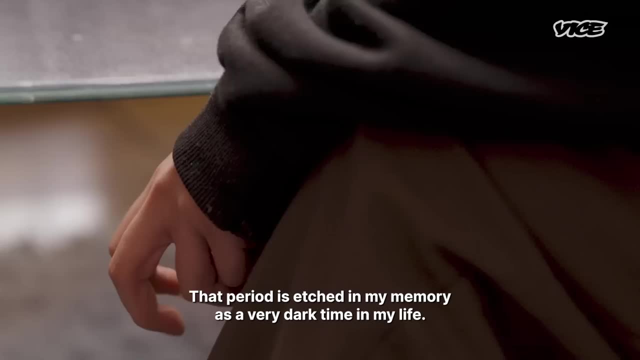 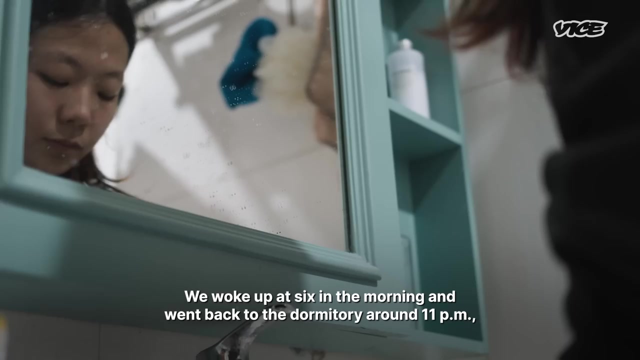 The teachers there were very fierce. They were the kind of students who would punish students and they would make students do a lot of homework. During that time I was in a dark night. I got up at 6 am and went back to my dorm at about 11 pm. 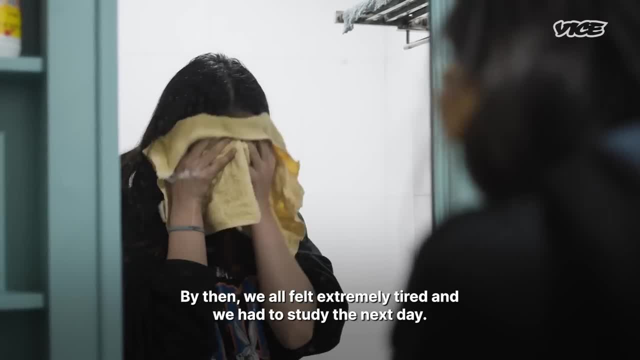 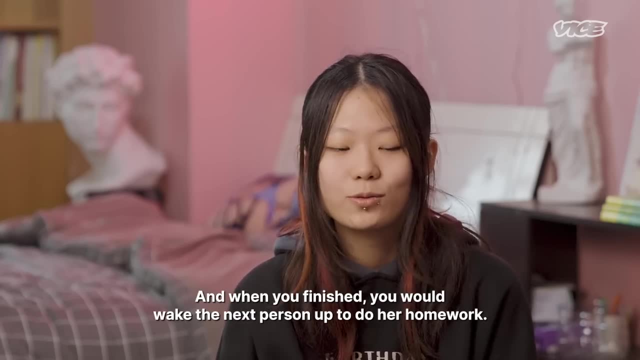 I finished my homework at about 12 am. Everyone was going to class the next day and they were all very tired. Some of the students would go to bed first and one of them would start writing homework. After he finished writing he would take a picture of the other student. 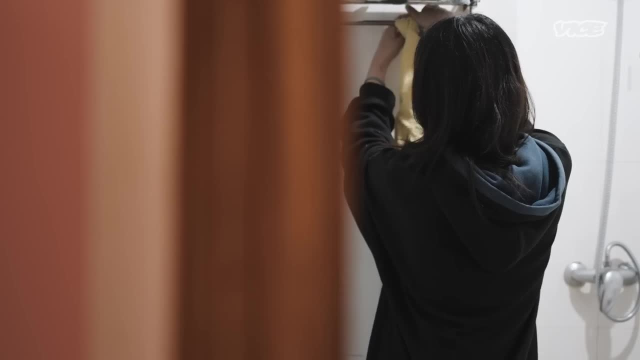 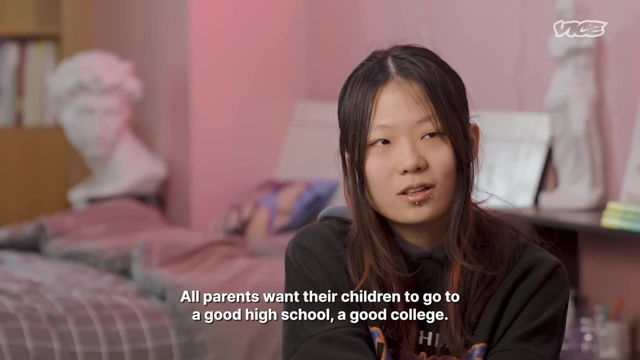 wake the other student up and then write the homework for the other student. Then he would write until around 3 am. Parents always want their children to be able to go to a good high school, a good university. Parents always want their children to be able to go to a good high school. 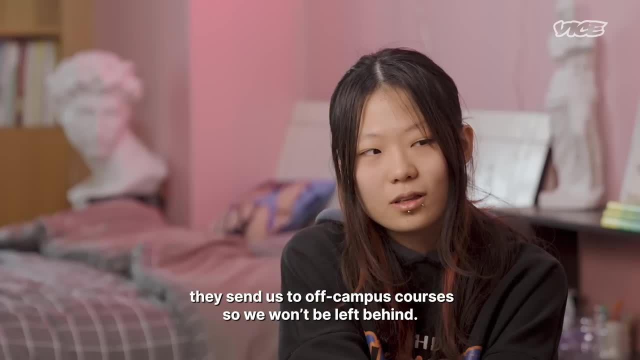 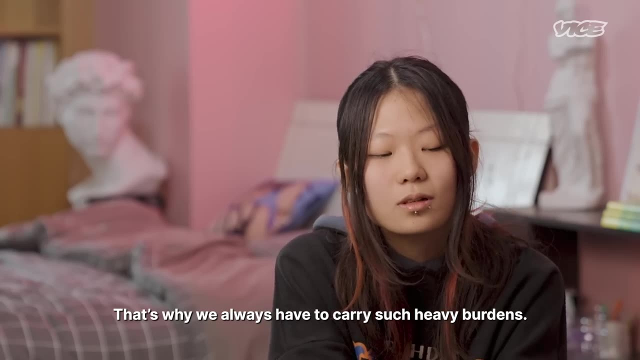 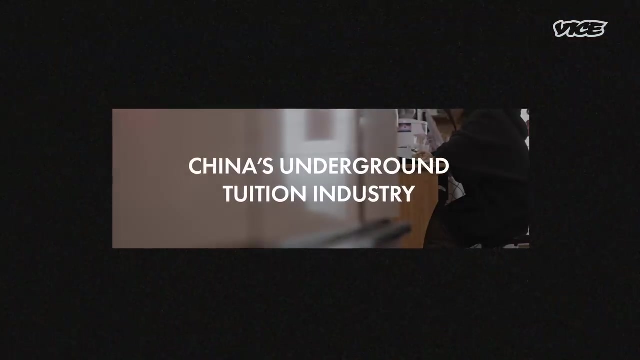 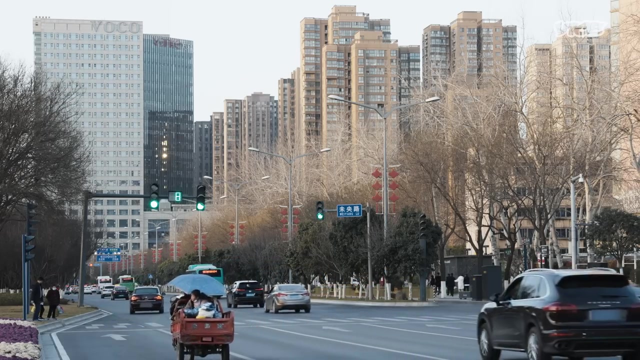 a good university. Parents always want their children to be able to go to a good high school so that they won't lag behind other people. If this is the case, the pressure on my children will be very high. In July 2021, the Chinese Communist Party announced its new double reduction policy. 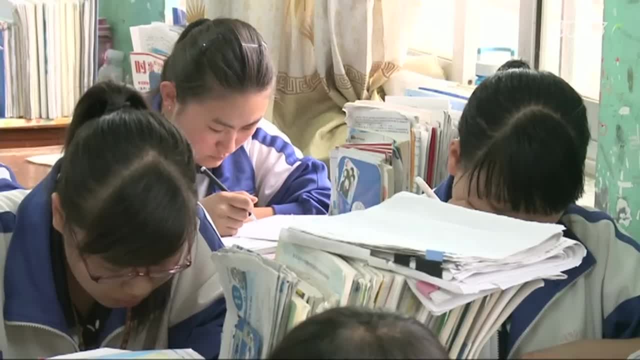 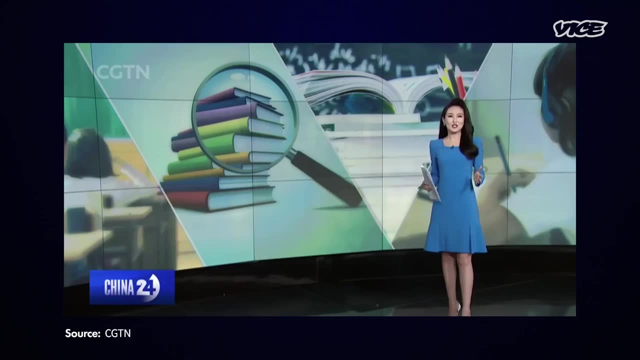 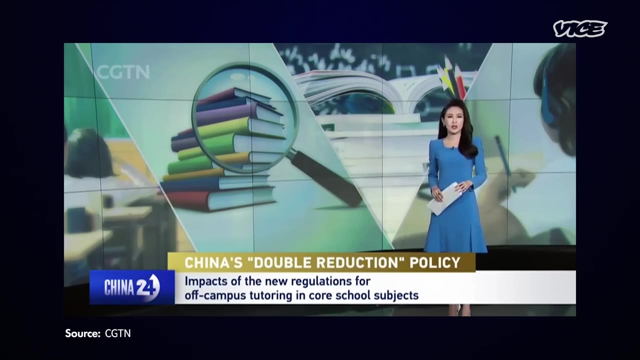 The new regulations aim to reduce pressure on parents and children by stopping excessive homework and banning certain types of off-campus tutoring. China has issued regulations for off-campus tutoring services, banning private firms from offering after-school training in core school subjects. Well, the move has raised concerns among both parents and private education institutions. 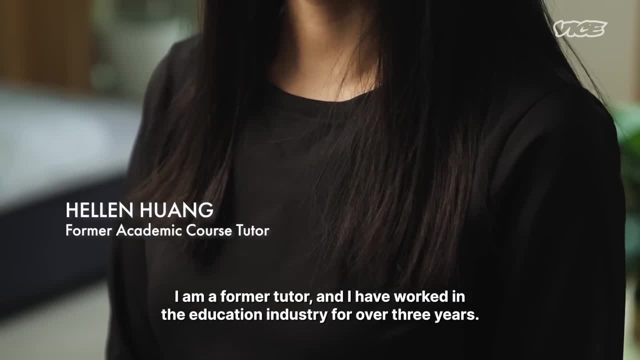 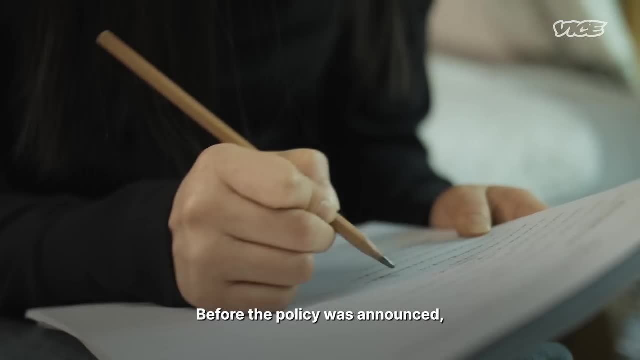 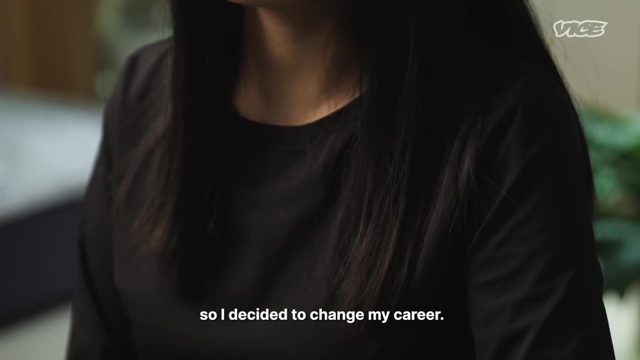 Prof Shiyun. I have been a teacher for nearly three years. I've been in the education industry for nearly three years. I started working in an office after the transition to a new job after high school. I was told some things before the double reduction policy was introduced. 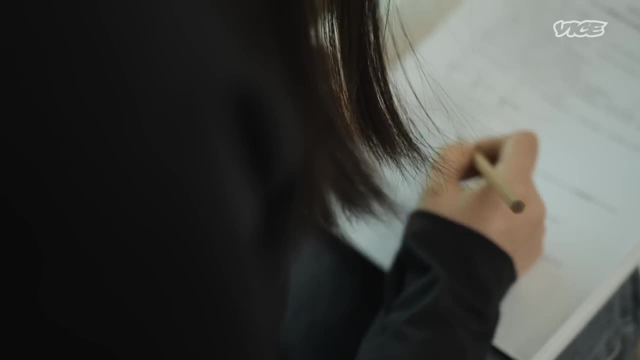 So I decided to switch jobs and go to a company. What does the double reduction policy entail? What does the double reduction policy entail? I think the study time for students and their everyday life is pretty tight. I think the double reduction policy entails that students don't have obvious works to do. 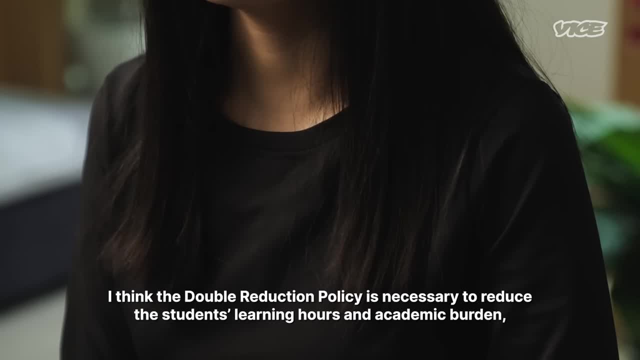 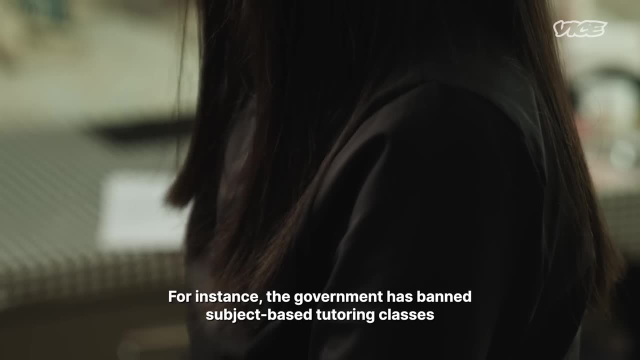 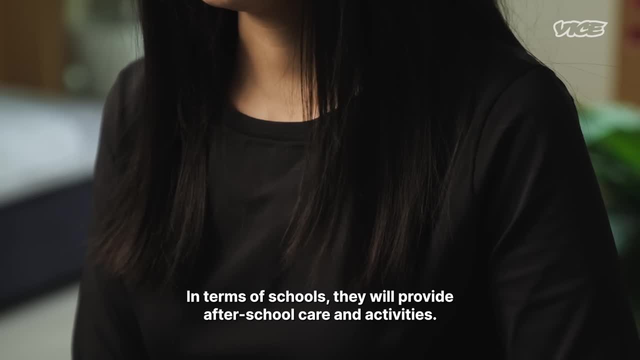 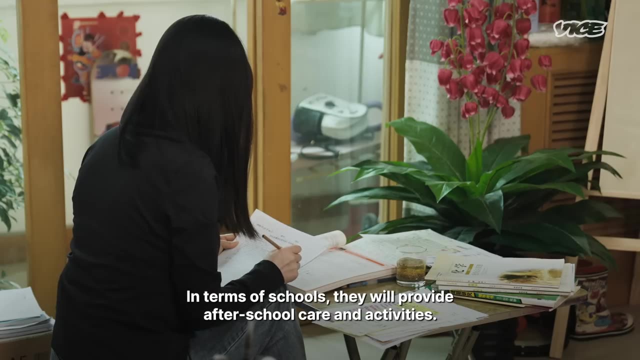 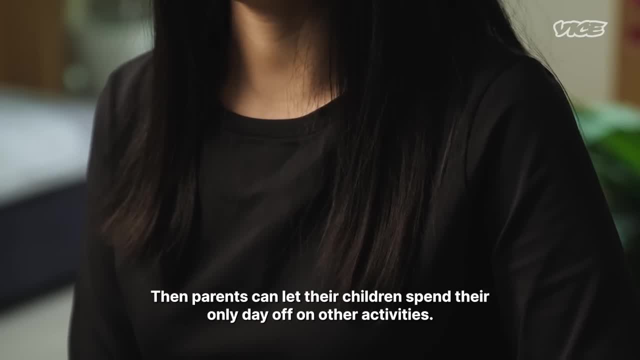 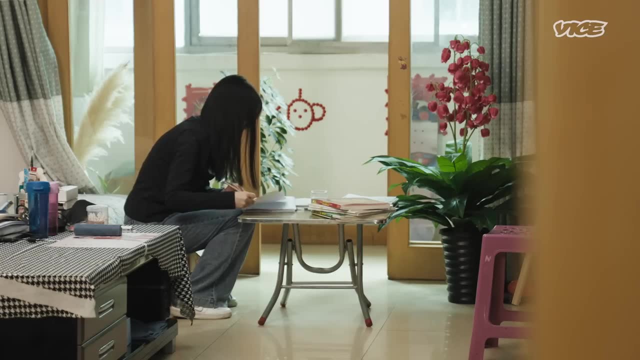 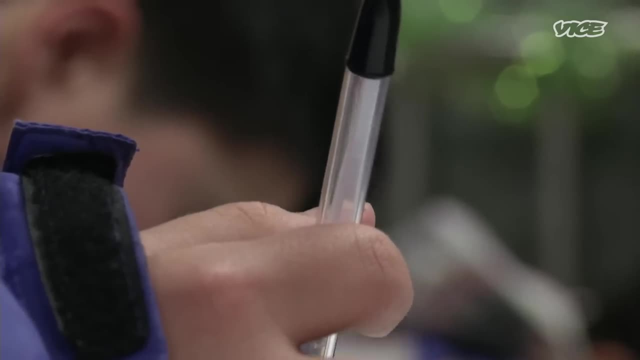 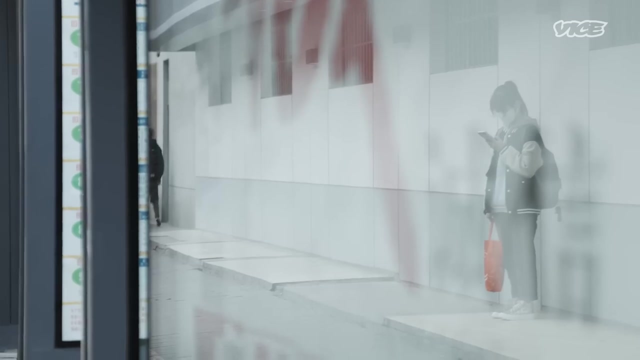 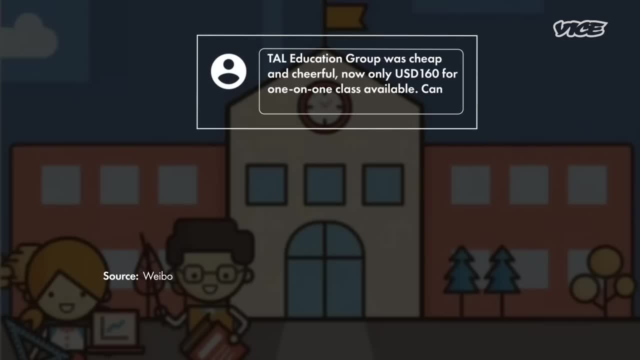 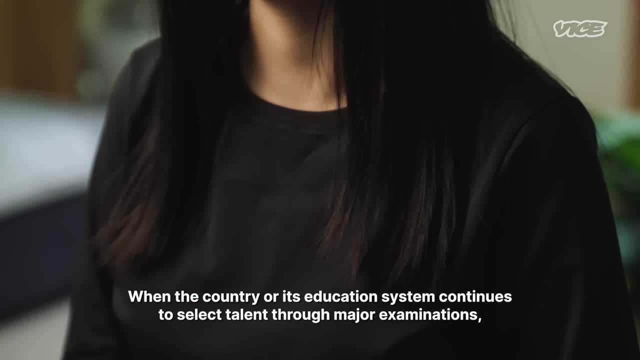 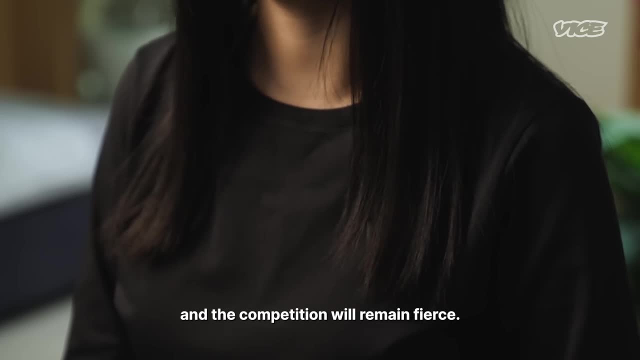 to reduce the burden of learning. to reduce the burden of learning, to reduce the burden of learning. I definitely hope that the kids' grades will be higher and their competitiveness will be stronger. So when parents are allowed to do so, they will invite their teachers to their homes. 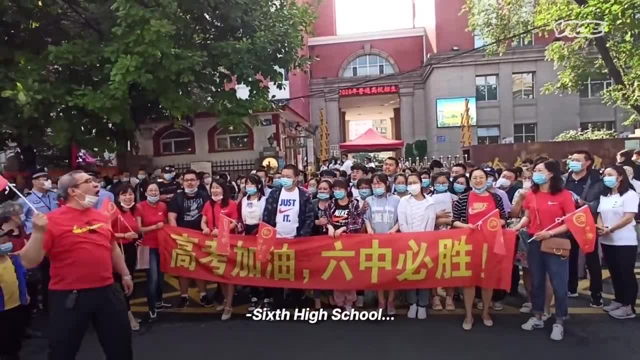 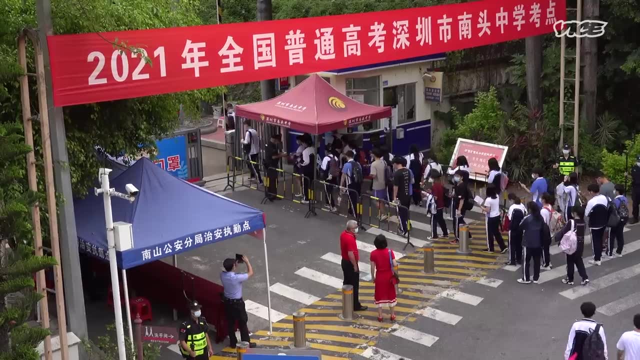 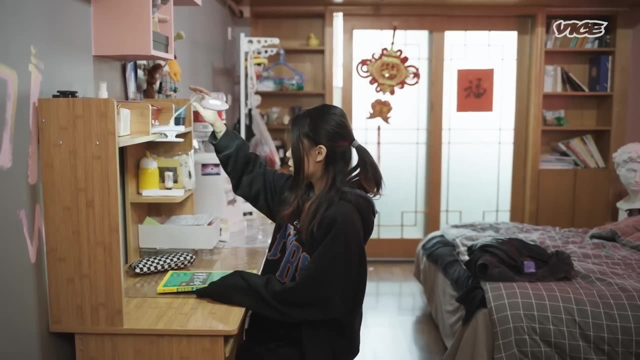 Our college entrance exams. We will win, We will win, We will win. In China, good academic scores lead to social mobility and the promise of a better life, especially for those from poor rural communities. But for parents like Daixu Qi's, 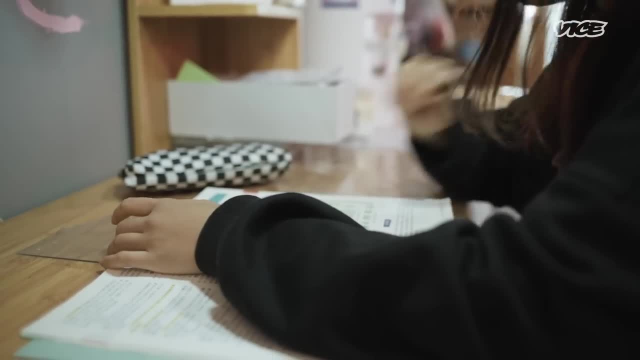 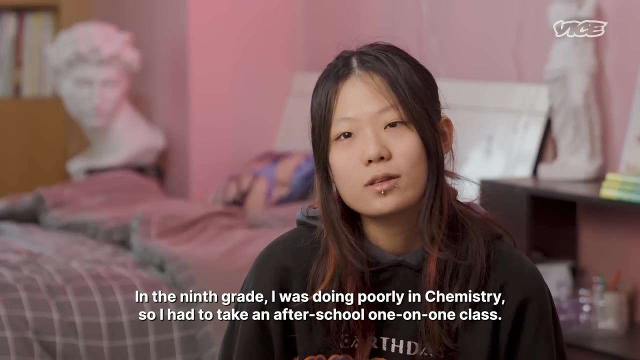 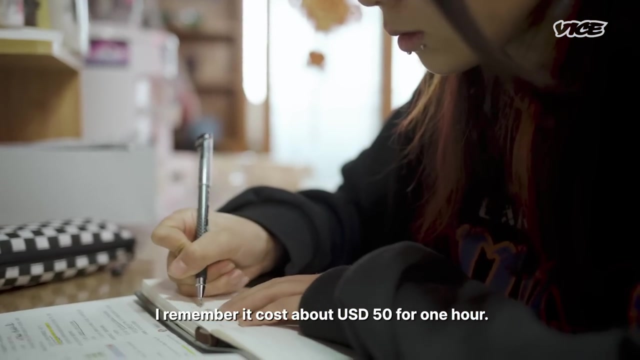 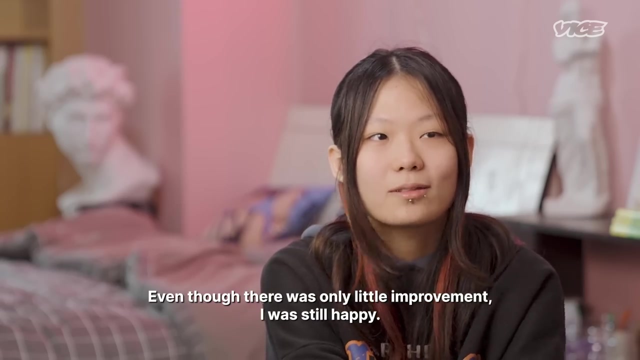 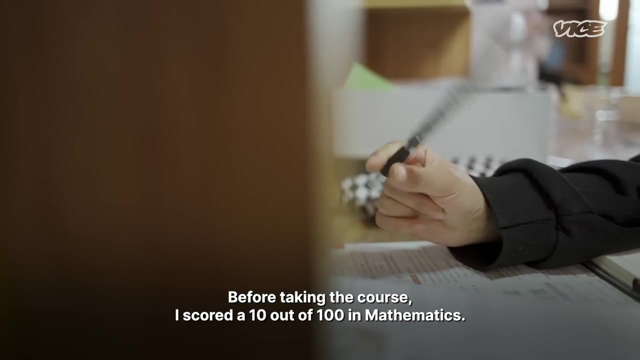 private tutoring is used as a way to ensure that a family's middle-class status will endure to the next generation. When I was a kid, I got 10 or so marks in math. That was the lowest score I ever got in my exam. 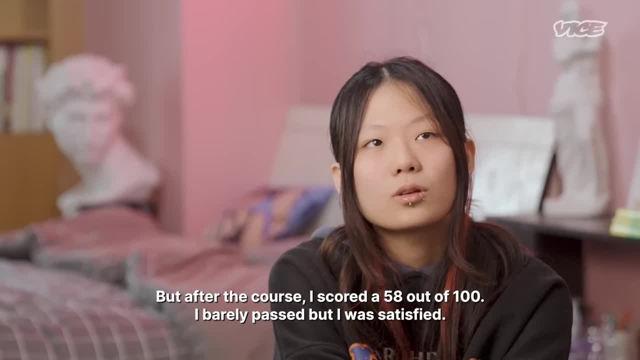 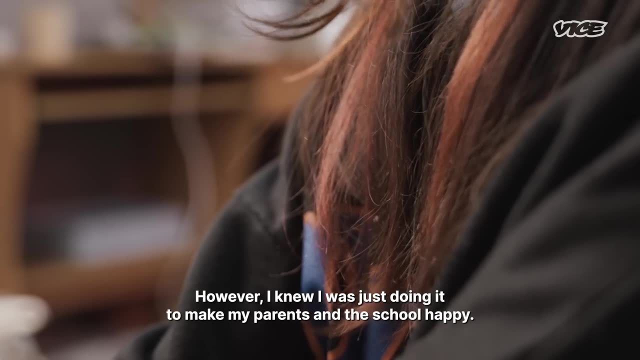 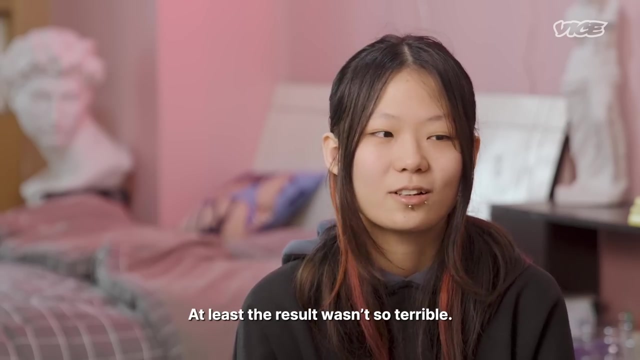 And then, after I got into the tutoring class, I got 58 or 60 marks. I was very happy, But the results I got in that situation made me want to make my parents and the school happy. I wanted to make my parents happy. 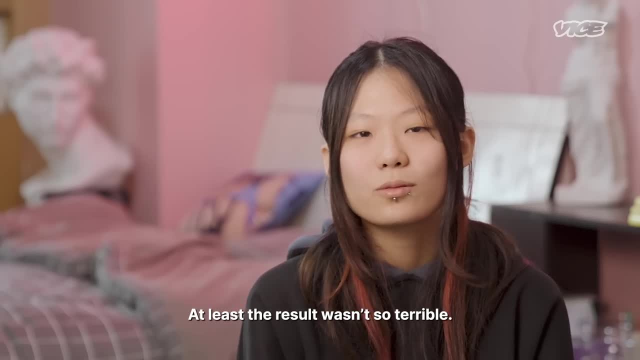 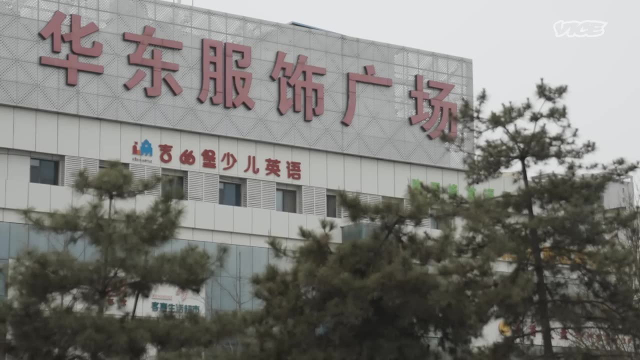 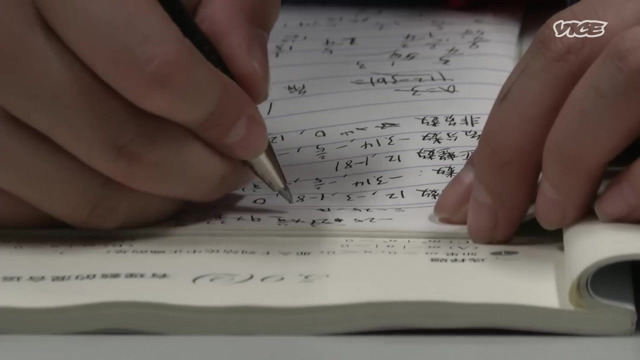 At least, I didn't want to look down on them. I couldn't stand it. There were an estimated 3 million education companies in China at the end of 2020.. The sudden overhaul sent tutoring companies into freefall. Tens of thousands of people lost their jobs. 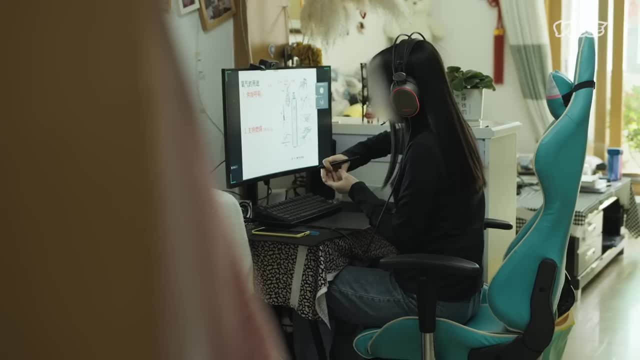 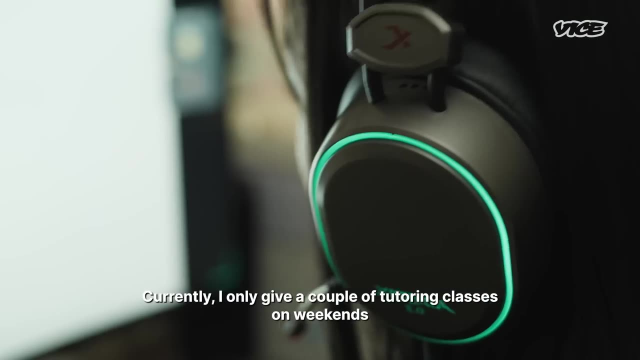 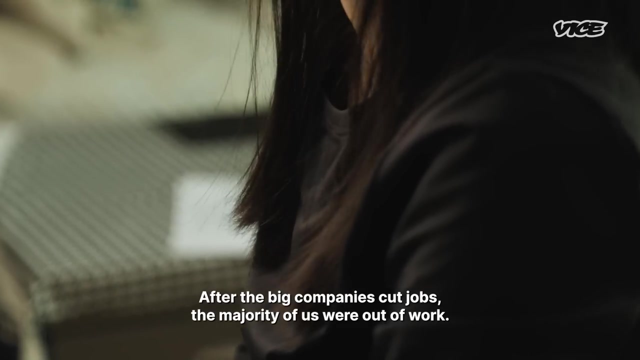 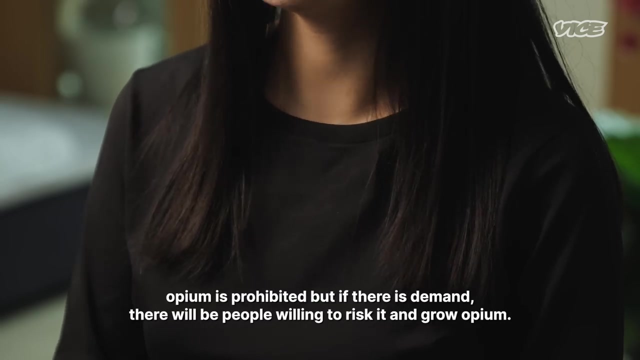 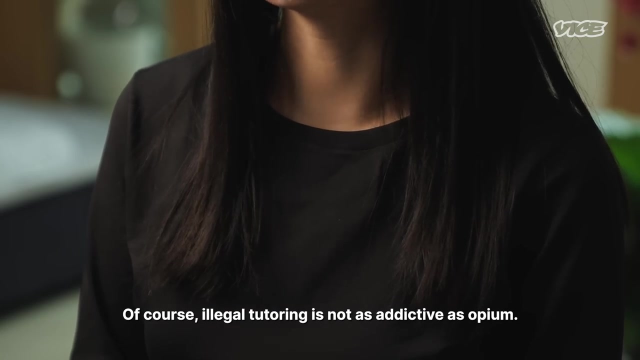 in the education sector overnight After I got to know those big companies. most of them were closed-off. For example, drugs are banned, But if someone really needs it, then someone will choose to stop it. Of course, tutoring is not as serious as drugs at the moment. 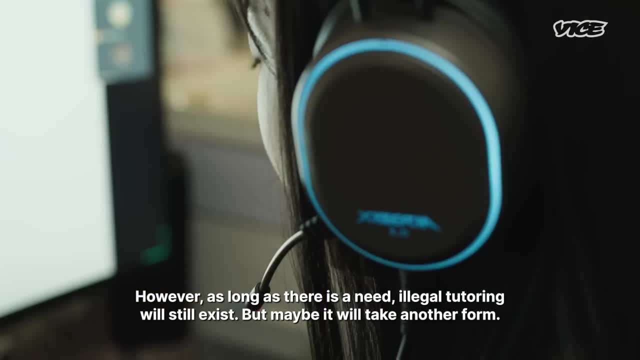 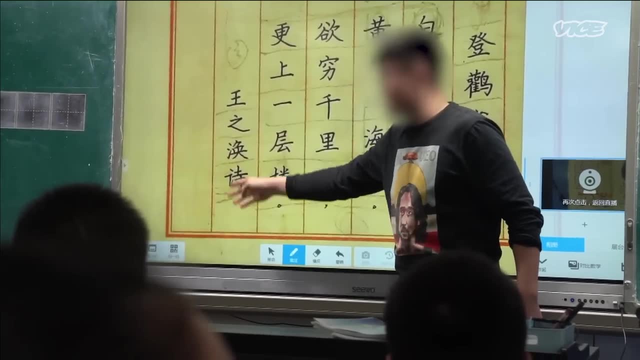 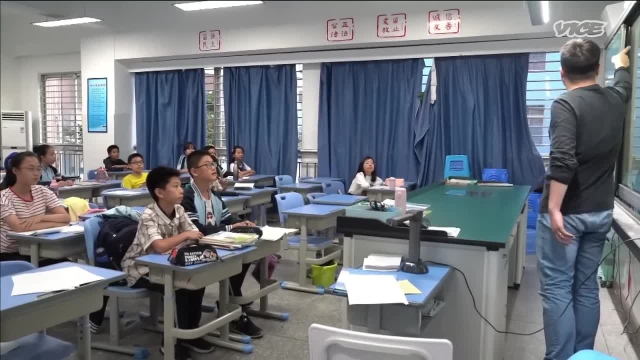 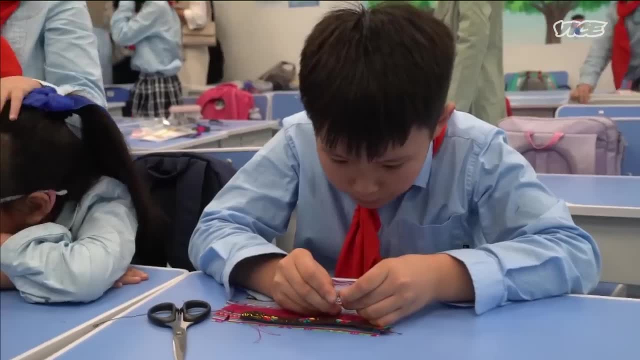 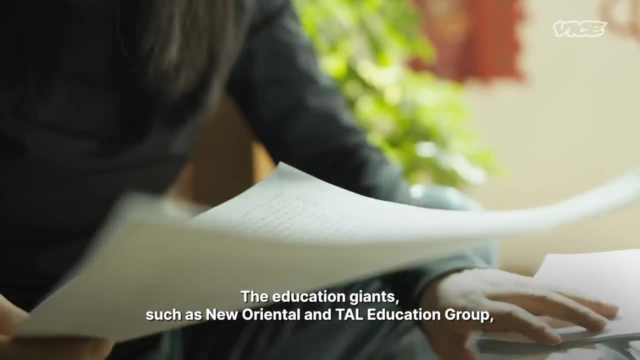 After the new regulations, tutoring companies were forced to either stop their primary and secondary school tutoring classes or pivot to new business models such as consulting services, off-campus care and non-core subjects like art. The big tutoring companies, such as the new school, 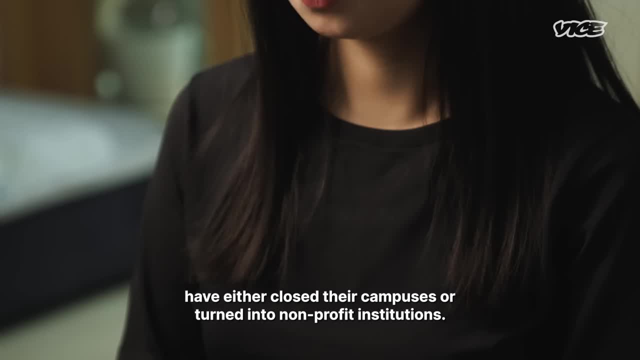 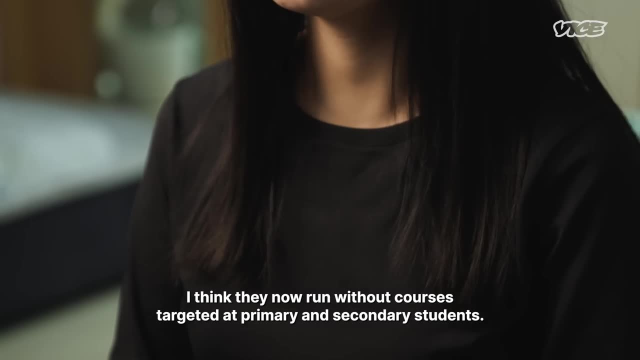 or the new school are gradually shut down or turned into non-profit institutions. The smaller local institutions, I think, will continue to exist for the time being, But as far as I know, most of them shut down all the primary schools because they don't want to risk it. 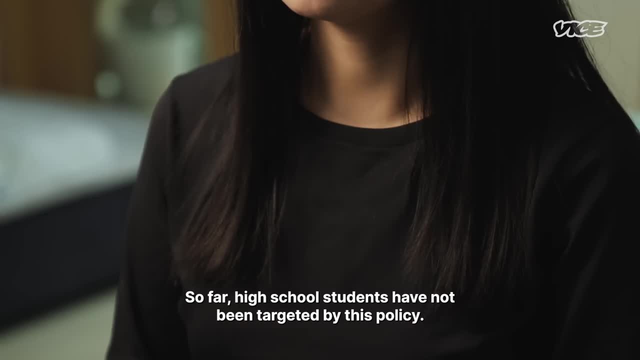 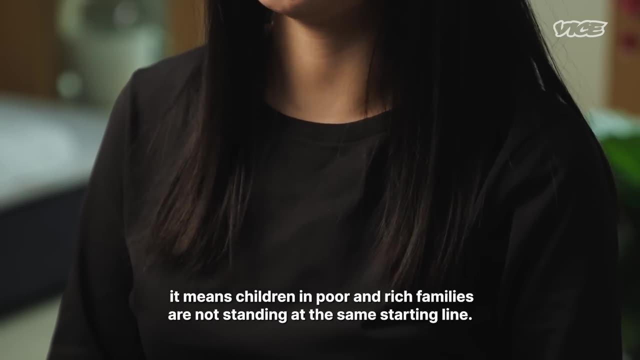 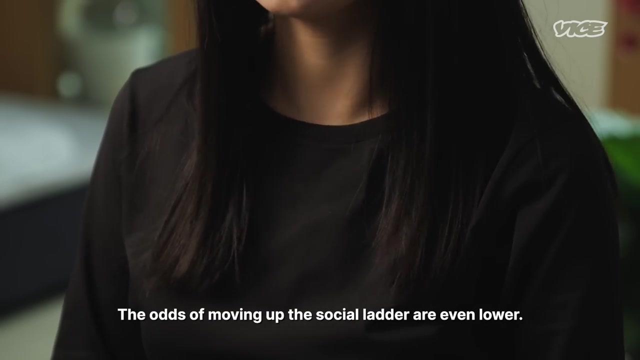 And then the high schools are still on the rise And policies are also allowed. Because, under the situation of inequality in educational resources, your starting line is different. It is really difficult to achieve some kind of class transcendence or change or, on a larger scale, 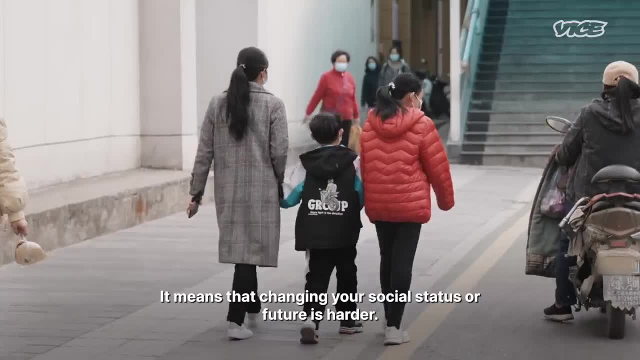 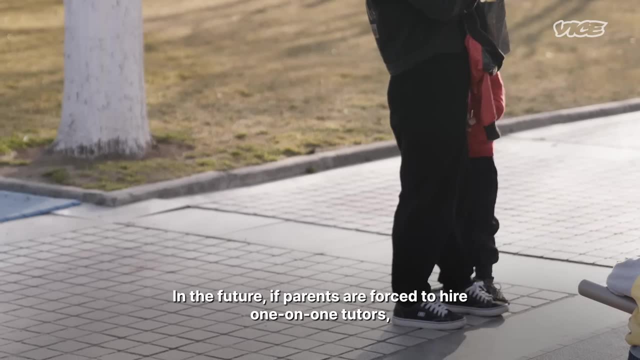 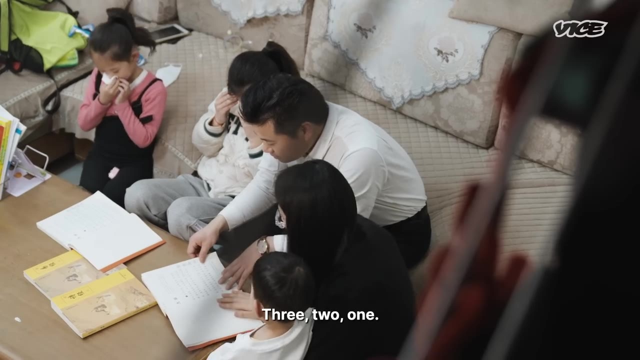 change your own level or your life in the future. And if it's really going to be one-on-one in the future, I think many families will have a hard time paying for it. Three, two, one: The way of the university is to be wise. 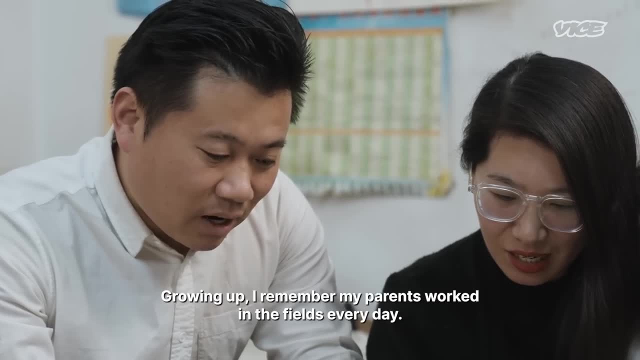 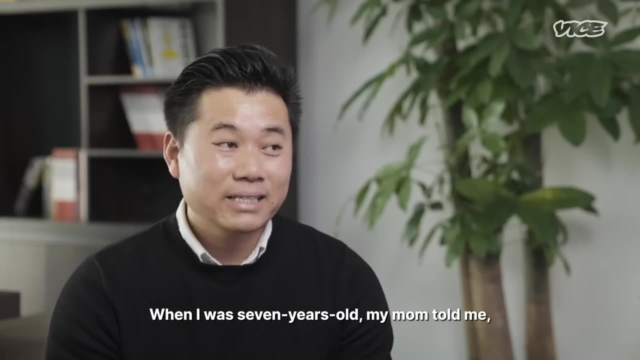 smart and kind. In fact, in my memory I remember that, you know, when I was seven or eight years old my mother would pat my shoulder and say: kids should go to school or you can't get out of the countryside. 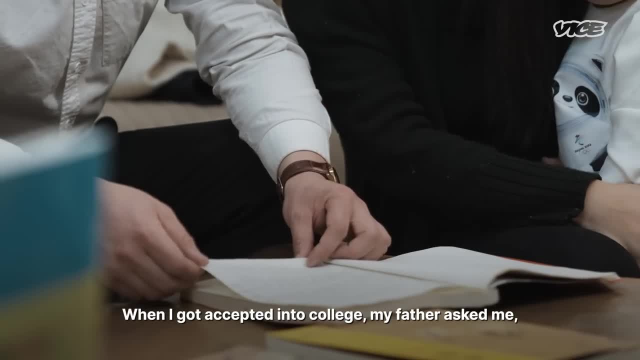 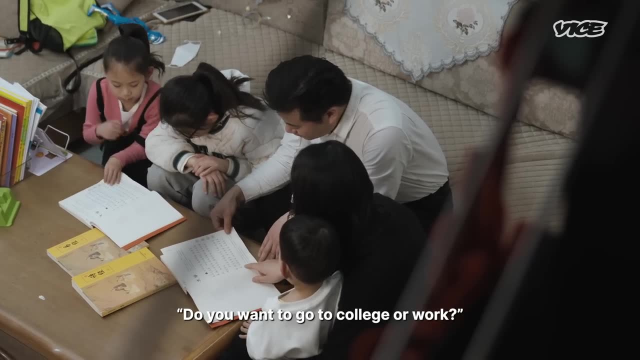 When I was very hardworking and went to college, my father actually asked me a question. He said: do you want to go to school or go to work? As a result, Mr Tan's father said: as long as you want to go. 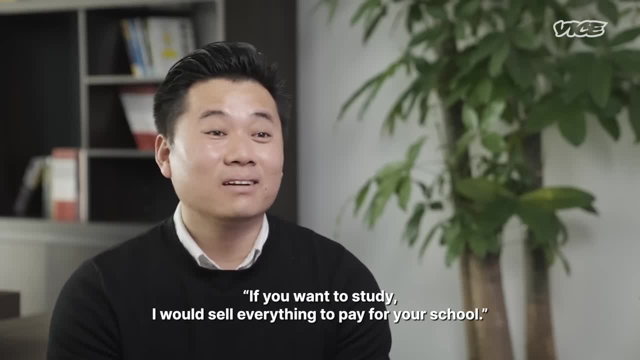 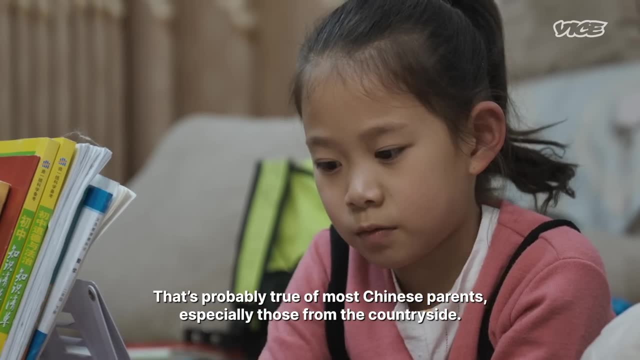 we will train you to be a good salesman. Maybe this is what many of our Chinese parents have in mind, And it's even more important to be a good salesman. That's it. Many of our rural parents in China want to change their children and their entire family. 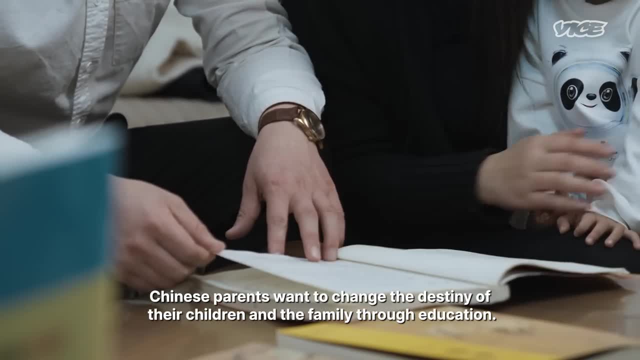 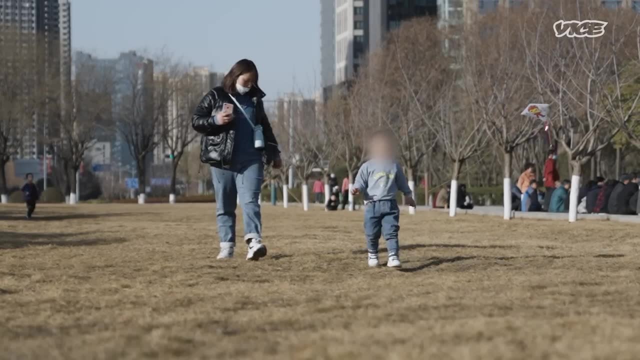 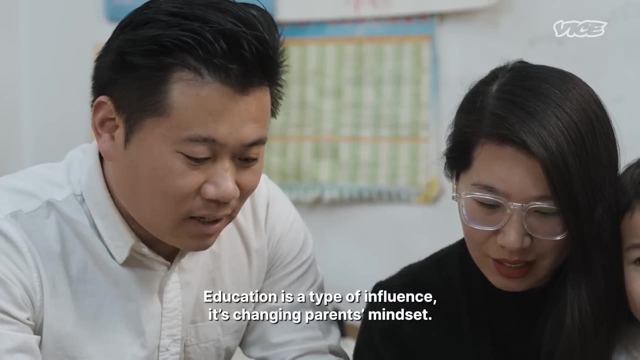 through education. As some anxious parents turn to the black market to find teachers, a new frontier in the Chinese education sector is attracting millennial parents. Education is an influence. First, it influences parents' thinking. You see some parents now, at least one or two. 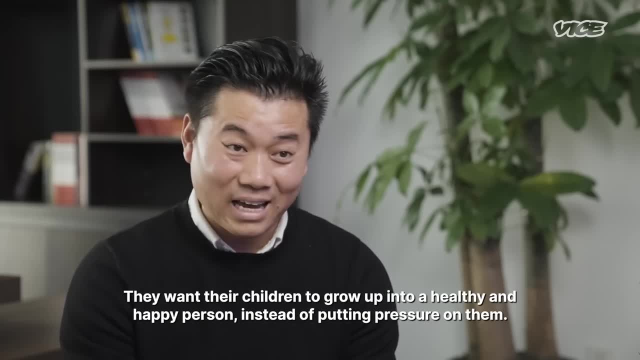 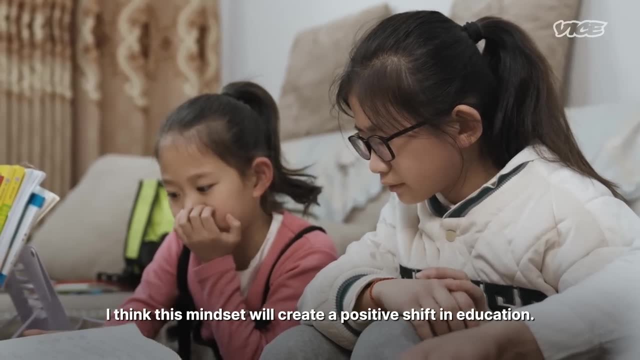 they already have this kind of idea. As long as my child is healthy, why should I put so much pressure on him, In fact, when he has this idea? actually, you find that education is really moving towards what I think is a positive change. 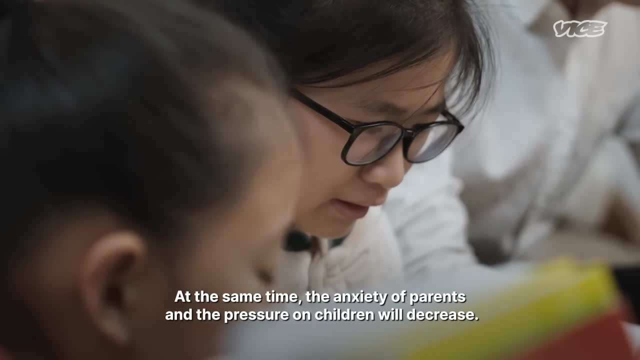 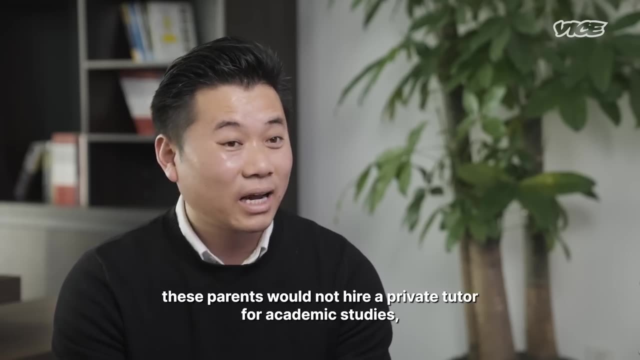 A positive change. This way, parents' anxiety will be lessened. At the same time, the pressure on the child will also be lessened. Even if the conditions allow, he will not invite private teachers to come to the house to tutor the children. 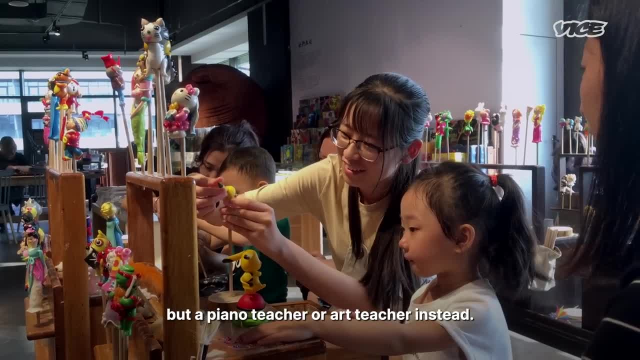 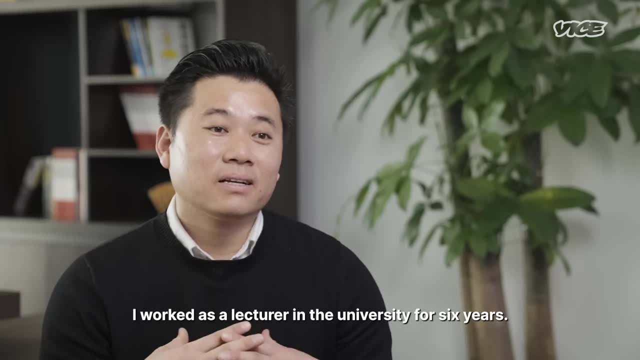 He may invite private teachers to play the piano for the children. He may invite private teachers to come to the house to tutor the children. The teacher came into our live broadcast room Today. Mr Tan brought home for everyone. I used to be a university teacher for six years. 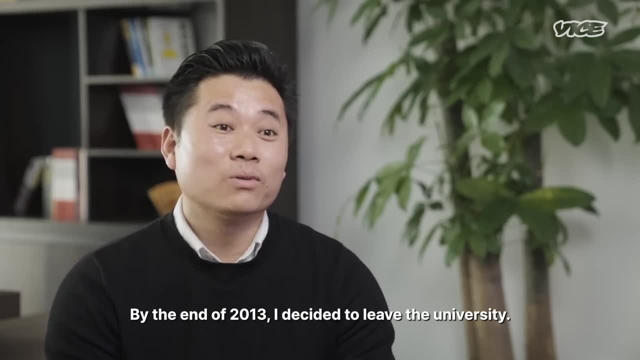 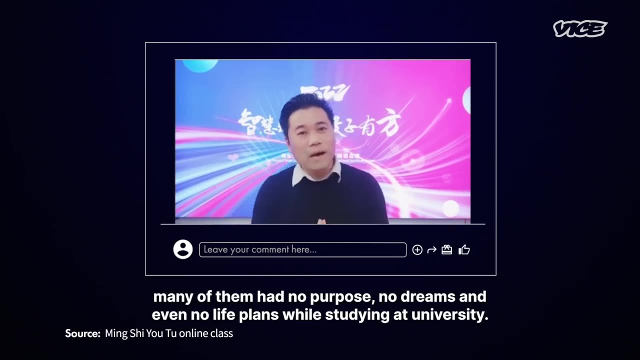 It was at the end of 2013 that I decided to come out of college. Many college students, although they worked very hard before going to college, but after going to college, there are still many children who have no direction, no dream. 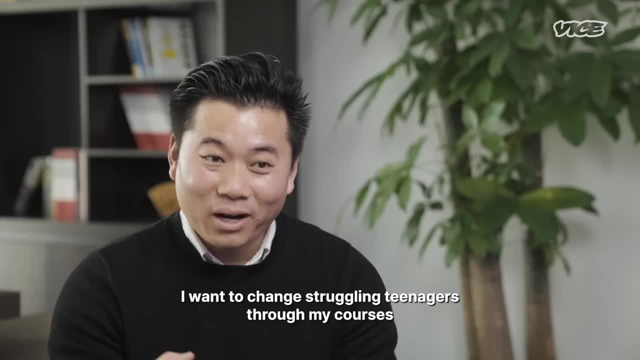 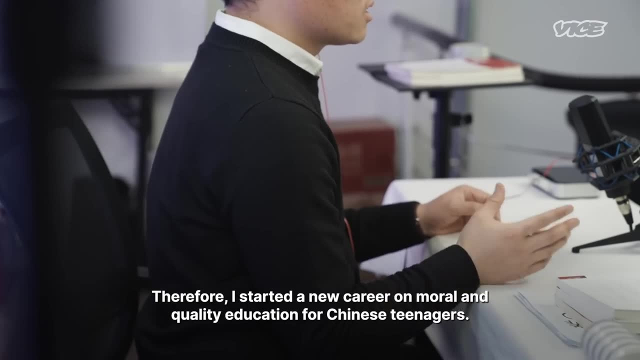 and even no life plan. I just want to influence them with a microphone, to make more children confident and strong In this way. I focus on the education and quality education of young people. The words of my father, you can write it down: 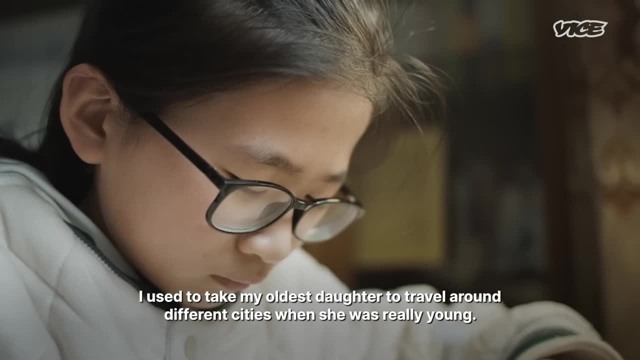 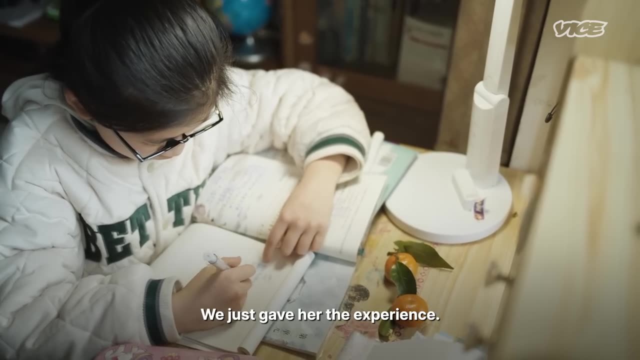 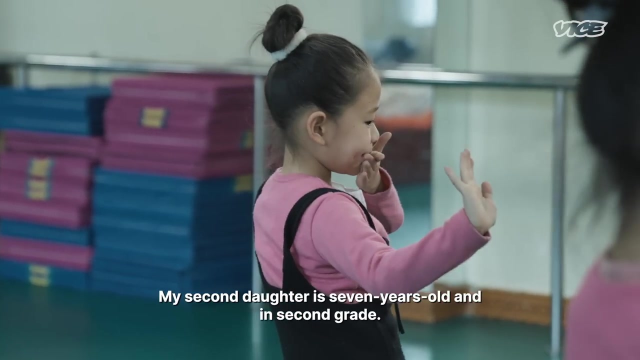 The high-speed rail. My eldest son has been following me to many cities since he was very young. Then we let him exercise One, two, three, four, five, six, seven, eight, nine, ten. My second son is in the second grade at the age of seven. 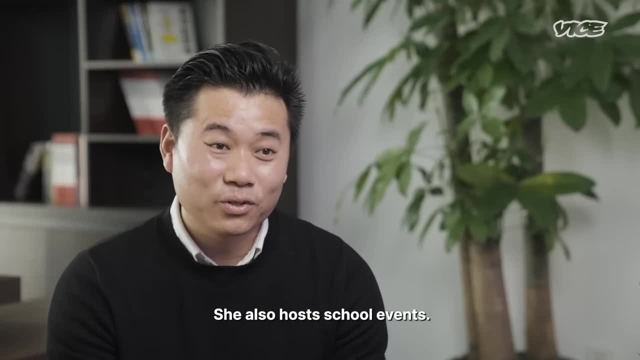 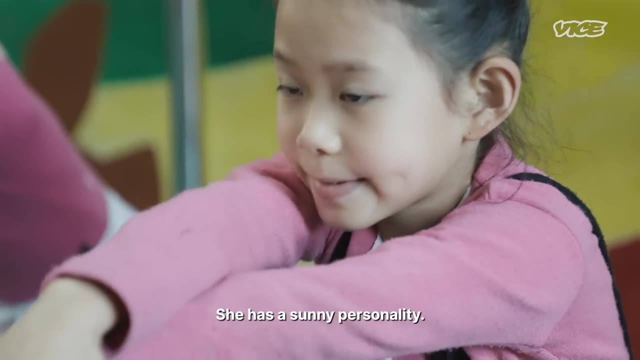 My second son. we usually train him to dance. Sometimes, for example, we organize an event for him and let him be a host. Let him dance. In fact, the child is also very sunny. Personally, I really don't have too much anxiety. 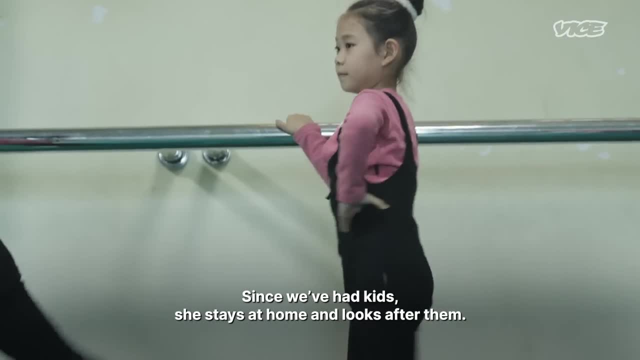 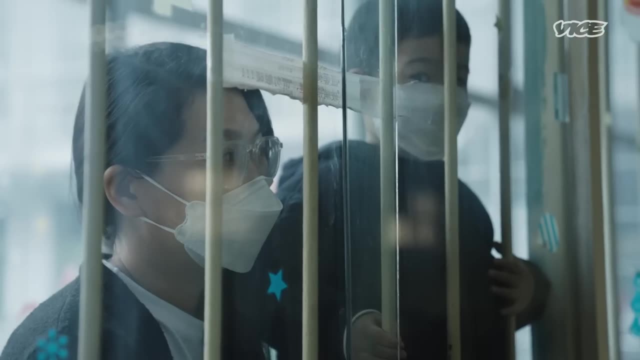 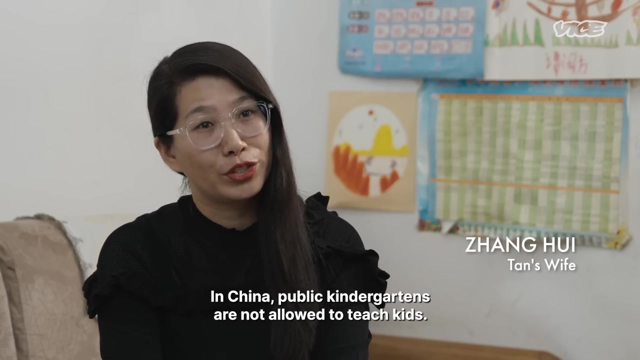 The child's mother may have some anxiety. So since I have a child, the child's mother basically does not go to work. She is focused on taking care of the child. My second daughter went to a public kindergarten. Public kindergartens are not allowed by the country. 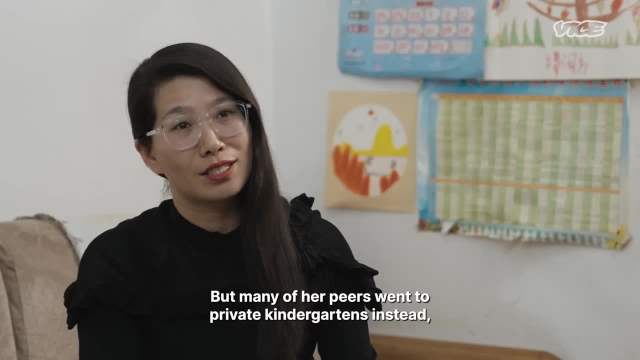 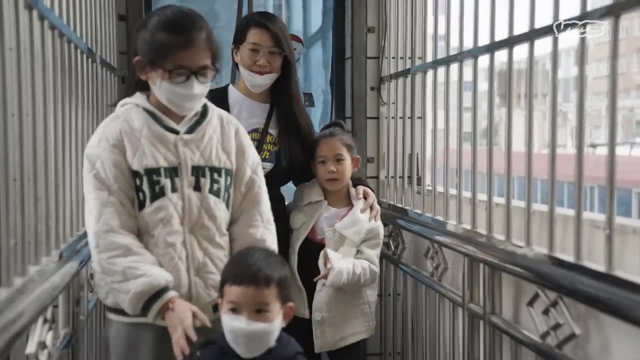 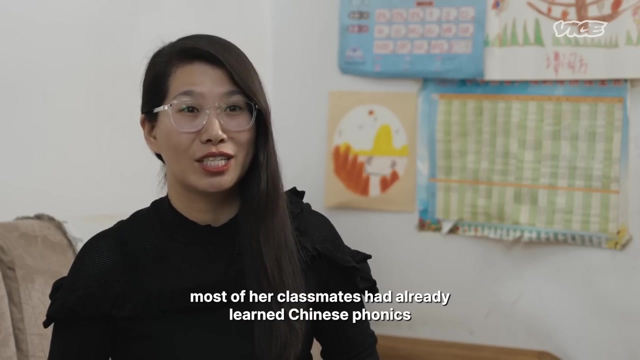 to teach knowledge. Many of her classmates go to private kindergartens. Private kindergartens teach a lot of knowledge, So before my child goes to primary school, she has no foundation. Her classmates may have learned a lot of knowledge. 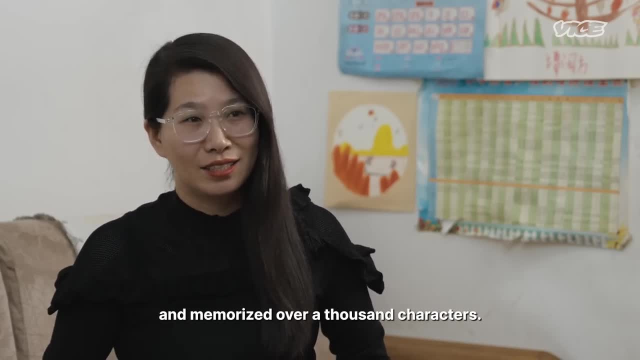 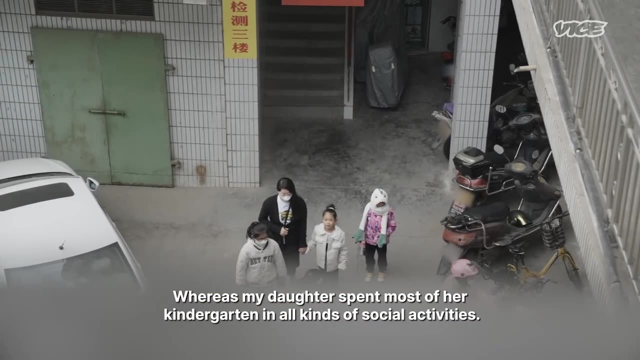 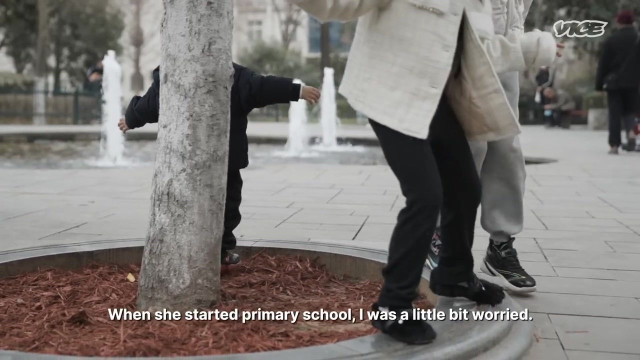 For example, to play the piano. Some of them know thousands of words, And so on. My child has been in kindergarten before primary school. She has been participating in social practice constantly. She has been in kindergarten for more than a year, So when I was in elementary school. 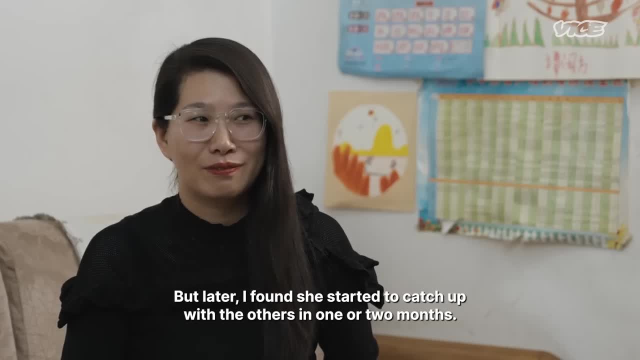 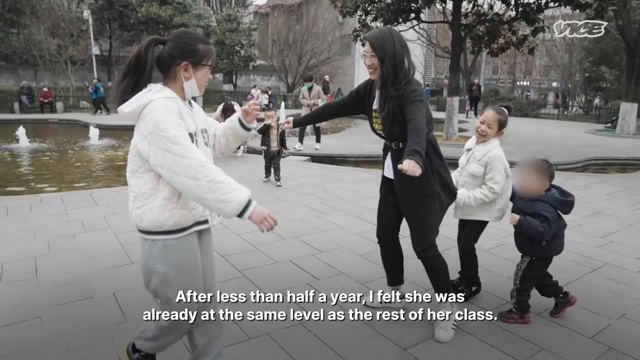 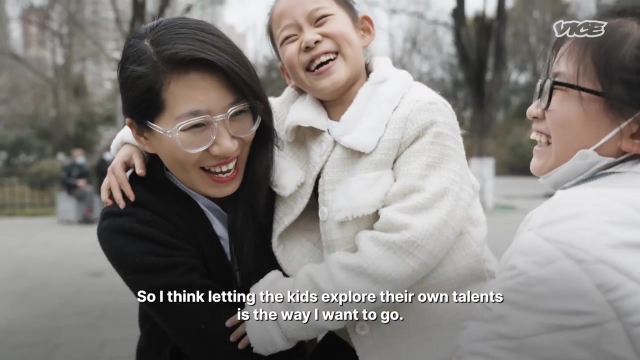 I was actually a little anxious at first, But I found that after using the time of one or two months, or less than half a year, I think the child basically reached the same level as the child. I think that to let the child play her nature. 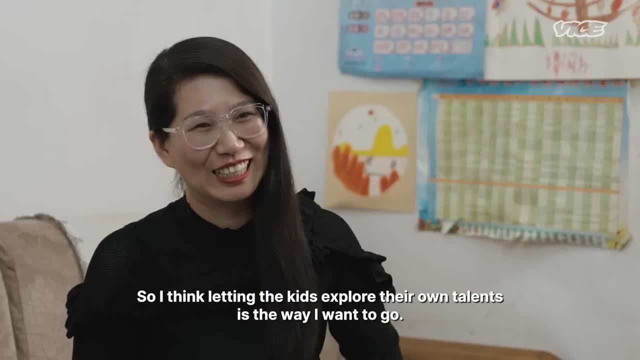 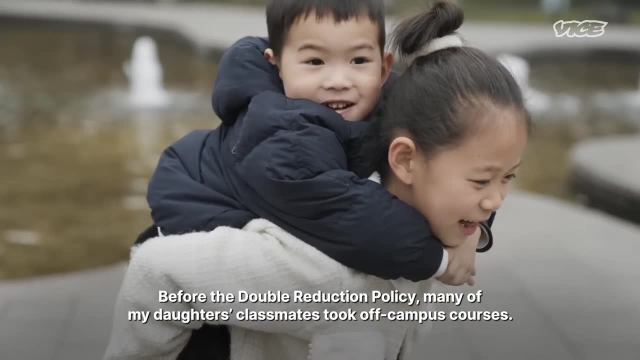 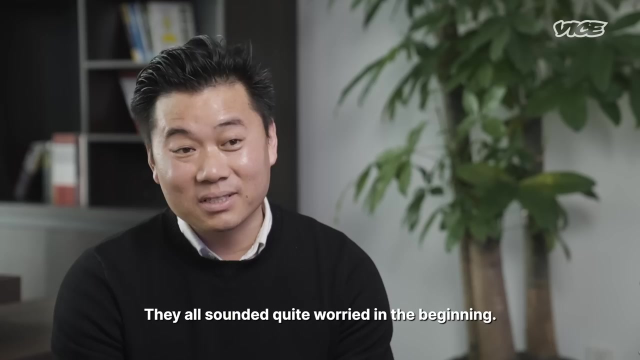 I think this is a path I want to take. Before primary school, many of my child's classmates were in private kindergartens. After primary school they- including some of our parents- they were discussing whether or not they can play the piano. 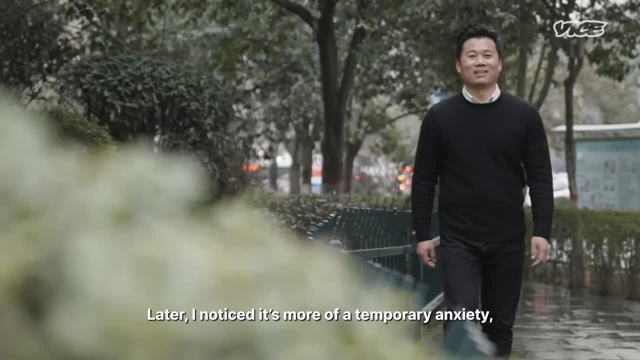 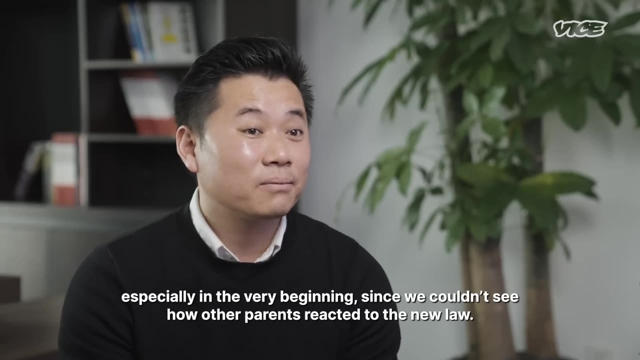 Right, Can the child play the piano, And so on. Then I found that everyone was just asking questions. They were a little anxious, They couldn't see the direction. But, for example, it's been a while since primary school. Everyone has seen. 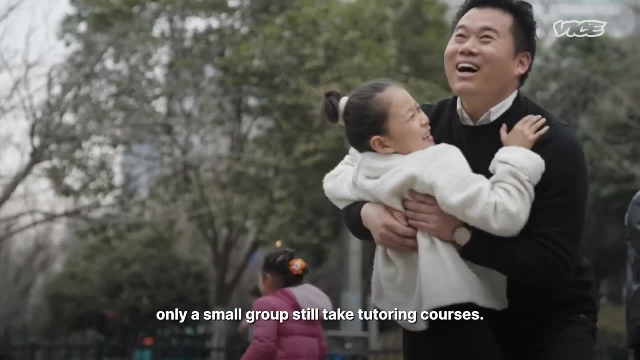 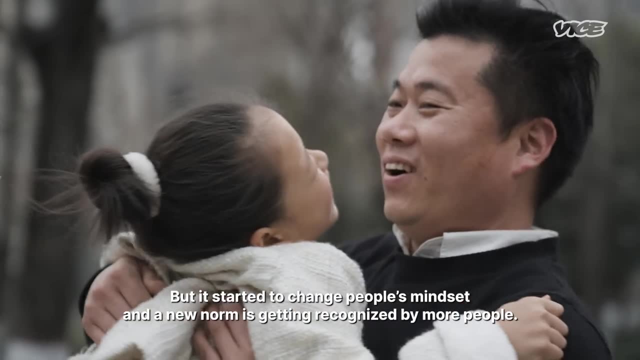 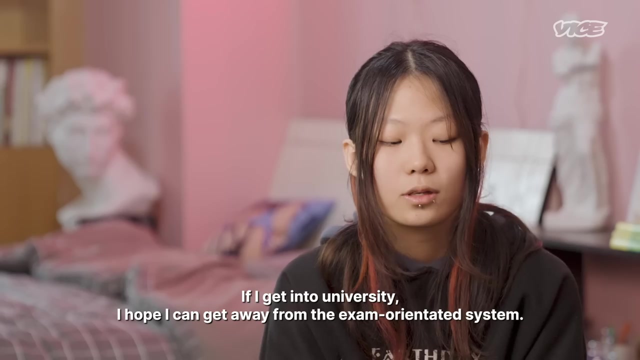 that, in fact, more people are now playing the piano. Of course, there are still some people who are playing the piano. Some people are playing the piano. The influence of this whole thinking is actually gradually recognized by more and more people. Then, when I came to those schools, 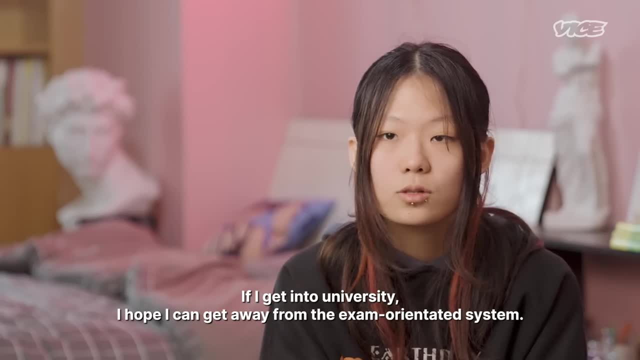 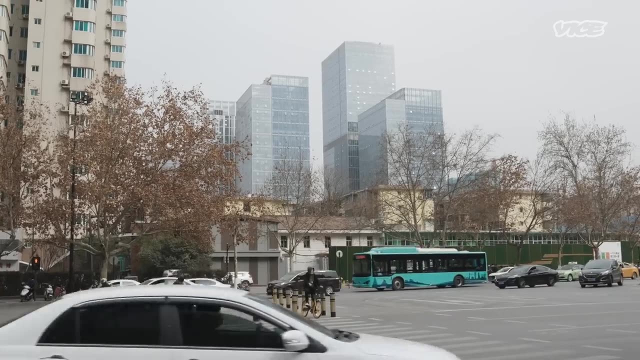 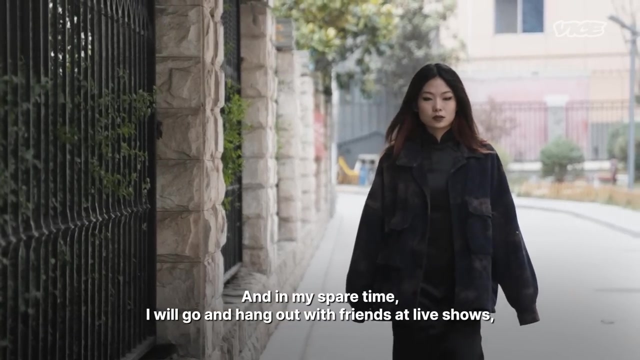 I was thinking more about jumping out of the past environment, that kind of hard world, And then when I was in the field, I was able to go to see performances with friends or to learn some musical instruments that I wanted to learn. For example, I wanted to do electronic music. 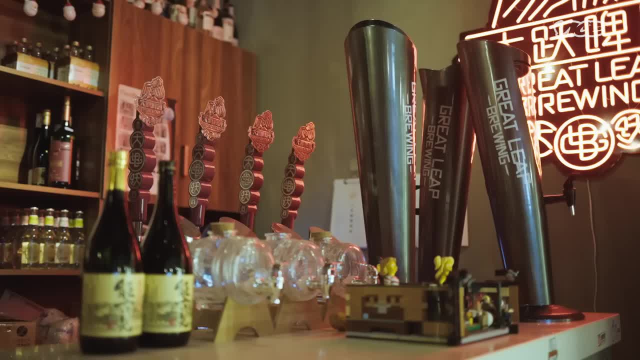 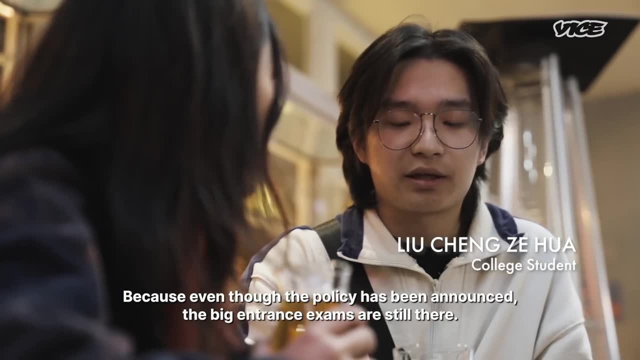 and then do what I wanted to do. The double-cut policy is actually not very effective Because even if it is cut again, you look at the high school entrance examination, the middle school entrance examination, it still has to be passed through the exam. 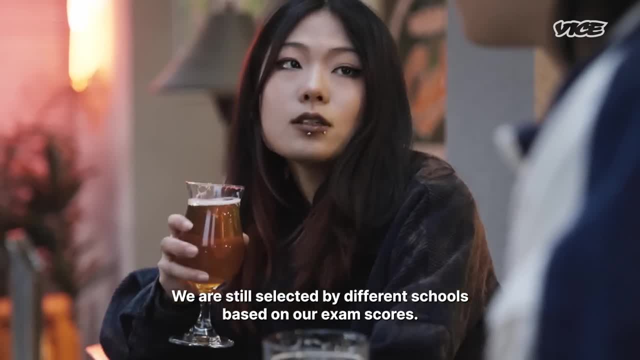 through hard things, to let you write a paper through your grades to get a good score, through your grades to get a good score, and then to assign you to a school, In this case, where the result doesn't change. I don't think it's going to work.